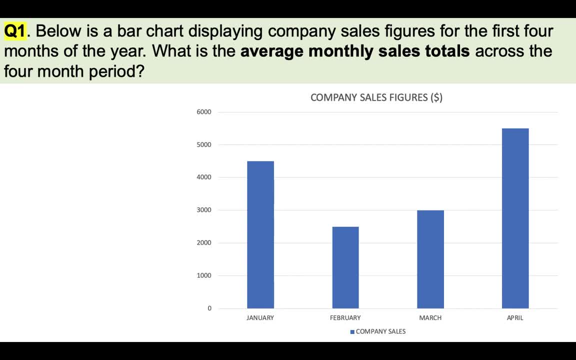 and find the average monthly sales totals, We need to follow two very simple steps. Step one: Add the total sales figures up across the four months And in this case it's $4,500 for January, $2,500 for February, $3,000 for March and then $5,500 for April, If we add. 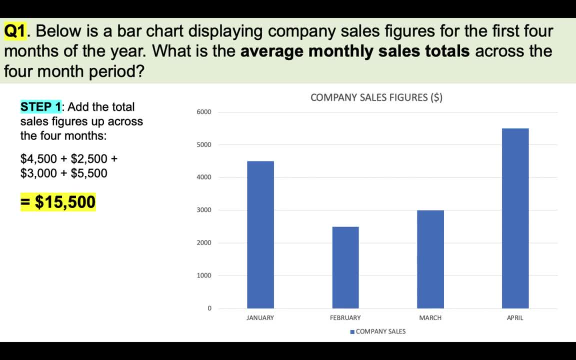 all of those up, then we get $15,500. And to get the average we follow step two, which is basically to divide the total sales by the number of months. In this case it's $15,500.. Divided by four, The correct answer is $3,875.. So very simple And this kind of bar chart. 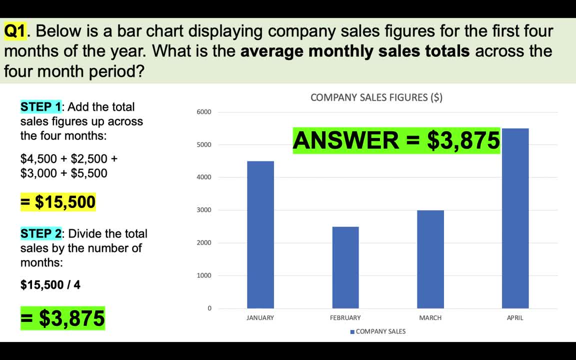 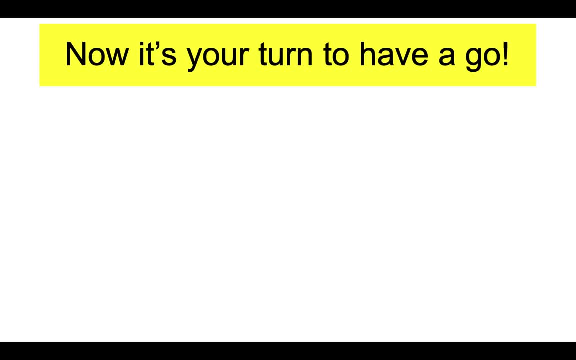 average calculation question is really common during maths exams and numerical reasoning tests And on that basis I would like you to have a go on to see whether you can answer it within a strict time condition. So please put your answer to question two in the comments. 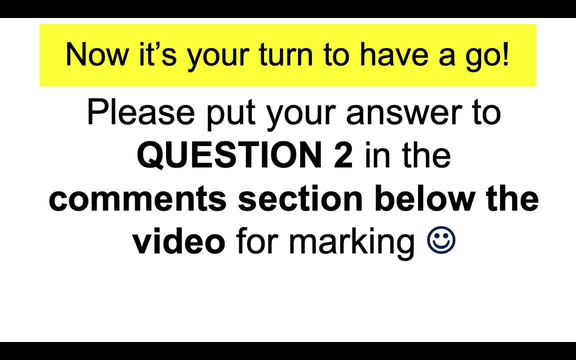 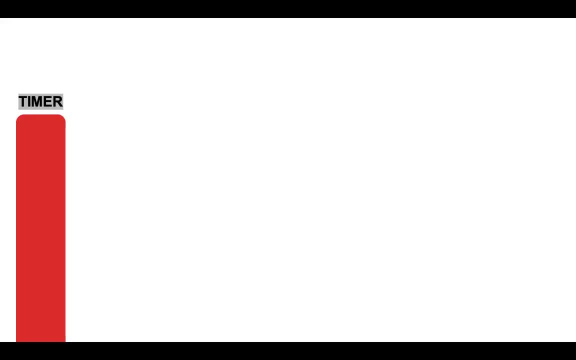 section below the video for marking. Now There is a question that I want you to try. There is a timer. You can use calculators if you want to, And that timer there is 30 seconds in total, So you don't have long to. 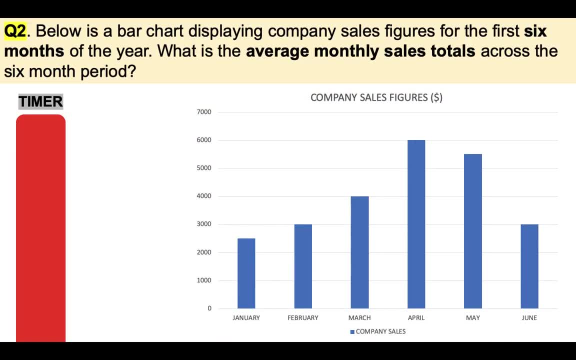 answer the question, And if you can answer this in 30 seconds, you are doing really well. If you find you need more time, please pause the video. It's important that you work through the question correctly. So question two. Below is a bar chart displaying company sales figures. 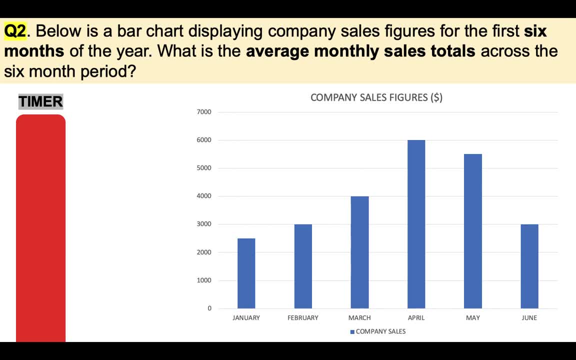 for the first six months of the year. What is the average monthly sales totals across the six month period? And you have the time. it takes the timer to go to the bottom to put your answer in the comments section below for marking. Here we go. 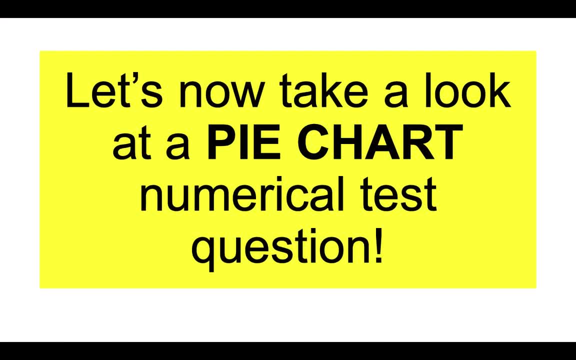 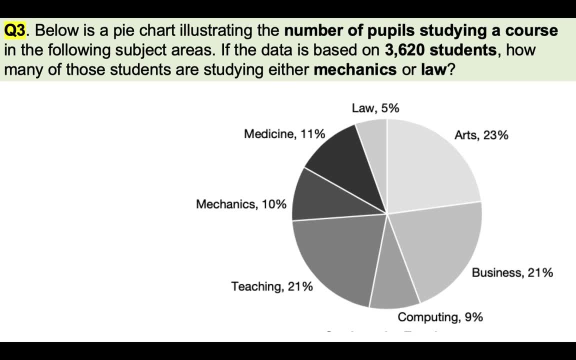 OK, Brilliant, Well done. OK, Let's now move on to a different kind of maths and numerical test question, which is pie charts. So question number three Below is a pie chart illustrating the number of pupils studying a course in the following subject areas. So we have law. 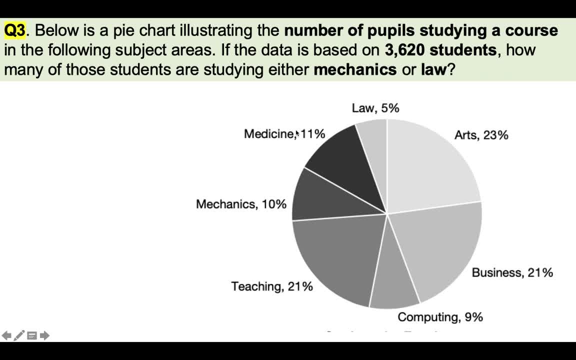 arts, business, computing, teaching, mechanics, the medicine, and then we have the percentages of students who are studying on each of the course. How, How many of those students are studying either Mechanics or Law. We can see here: Mechanics is 10% of that total and Law is 5%. 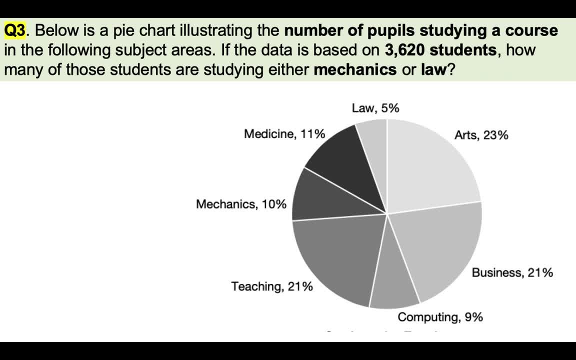 We need to calculate 15% of 3620 students. to get the answer, We follow again some simple steps. Step 1. Calculate how many students equals 1%. Well, if 3620 is 100%, we divide it by 100 to get 36.2.. 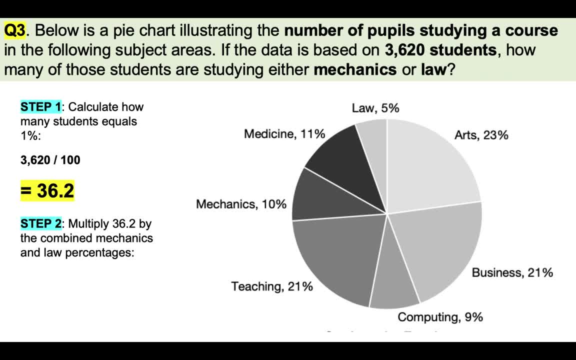 That's 1%, And then all we need to do is multiply that 1% by the combined Mechanics and Law percentages, which, as we already know, is 15.. So 36.2 multiplied by 15 gives us 543 as the correct answer. 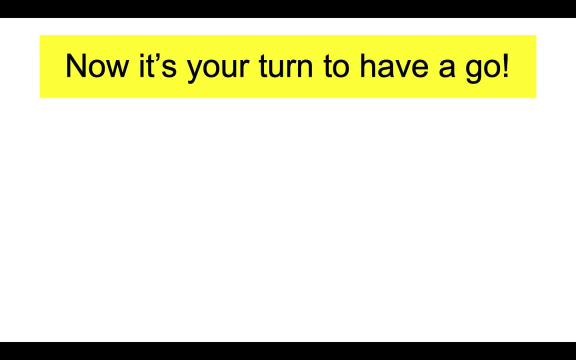 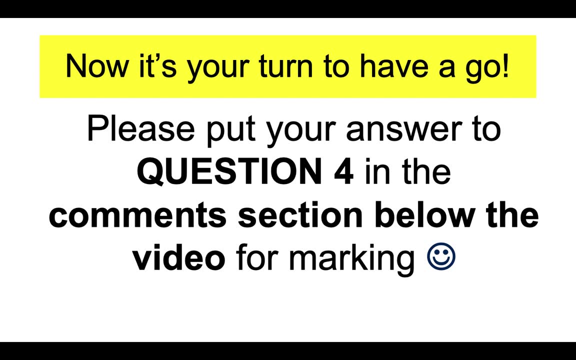 Very simple when you follow those two steps. So now it's your turn to have a go at a pie chart test question. Please put your answer to question 4 in the comments section below the video for marking. Again, you have a timer And the question is…. 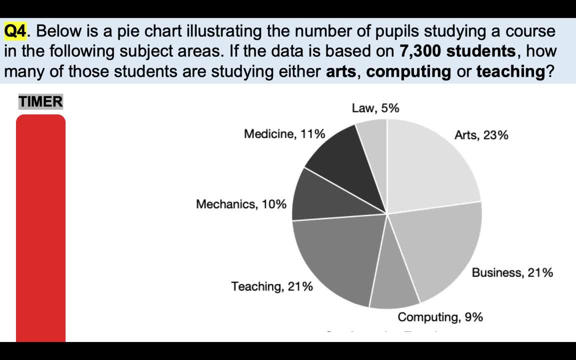 Below is a pie chart. It illustrates the number of pupils studying a course in the following subject areas. If the data is based on 7300 students, how many of those students are studying either Arts, Computing or Teaching? Here is the timer. 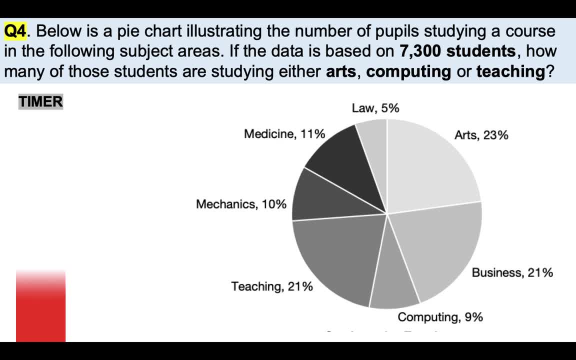 The answer is… 1., 2., 3., 4., 5., 6., 7., 6., 7., 8., 9., 10., 11., 12., 13., 14.. 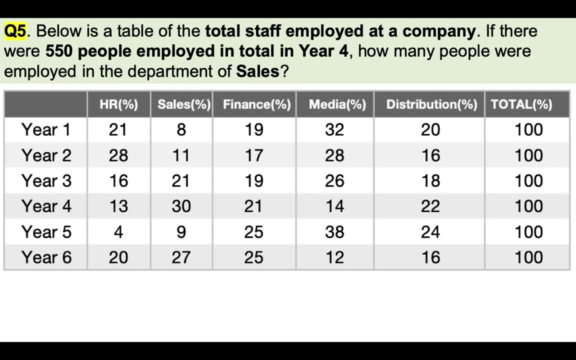 15., 16., 17., 18., 19., 20., 21., 22., 23., 24., 24., 25., 25., 26., 26., 27., 28.. 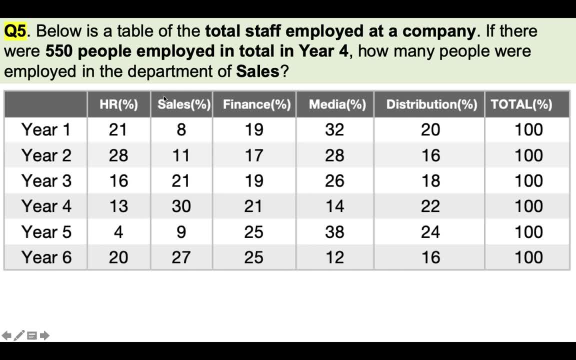 28., 29., 29., 30., 31., 32., 32., 33., 34., 35., 36., 36., 37., 38., 38., 39., 39.. 40., 41., 42., 42., 43., 43., 44., 45., 44., 45., 46., 46., 47., 48., 49., 50., 51.. 52., 52., 53., 52., 53., 53., 54., 54., 55., 56., 57., 58., 59., 60., 61., 62., 62.. 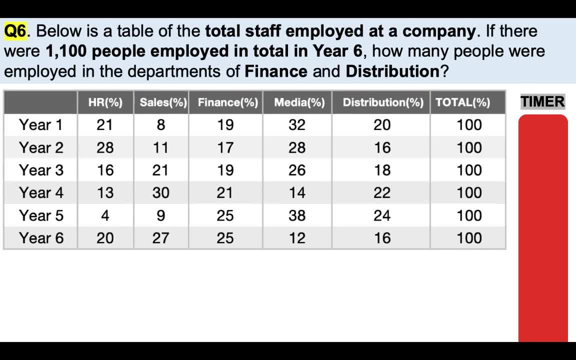 63., 63., 64., 65., 66., 67., 68., 68., 69., 69., 70., 71., 72., 72., 73., 74., 74.. 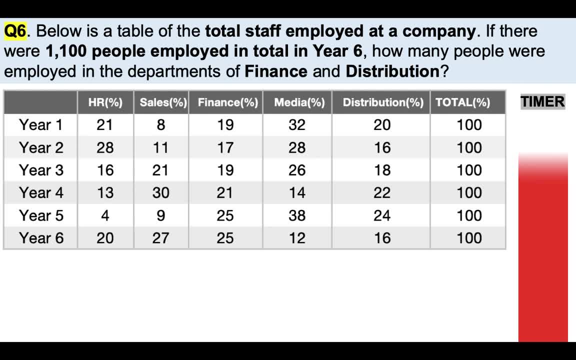 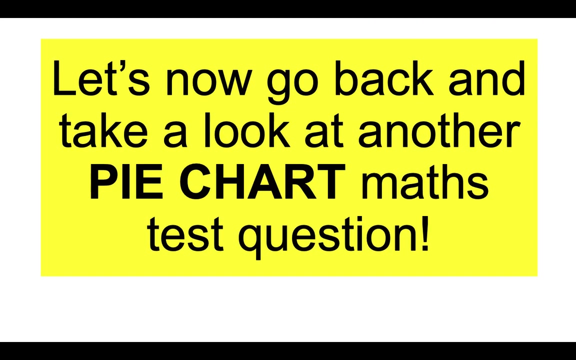 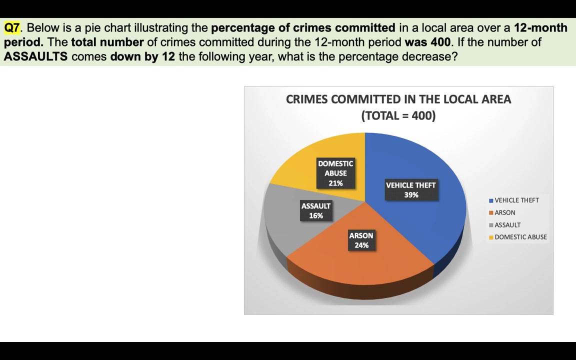 75., 77., 76. 75. 76., 77., 68., 68. period. Now, the total number of crimes committed during that 12 month period was 400, as indicated here on the top of the pie chart, And the question is if the number of assaults comes. 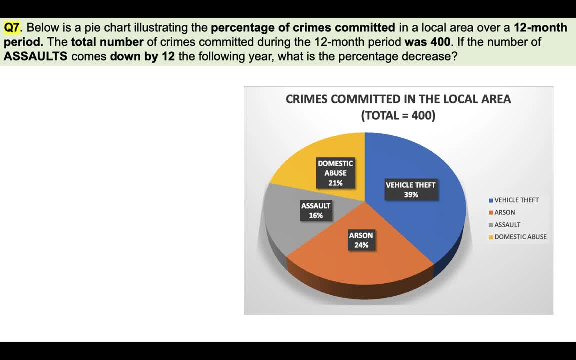 down by 12 the following year. what is the percentage decrease? So we have to calculate percentage decrease, which is not easy unless you follow this process. So we are focusing here on assaults. It's currently at 16% And we have to find out if it comes down by. 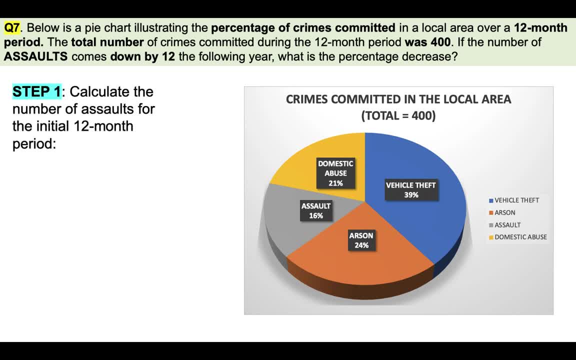 12 the following year. what is the percentage decrease? So, step one: calculate the number of assaults for the initial 12 month period. So it's 16% of 400. And to calculate that all we need to do is 400 divided by 100, for the 100% multiplied by 16, and that equals: 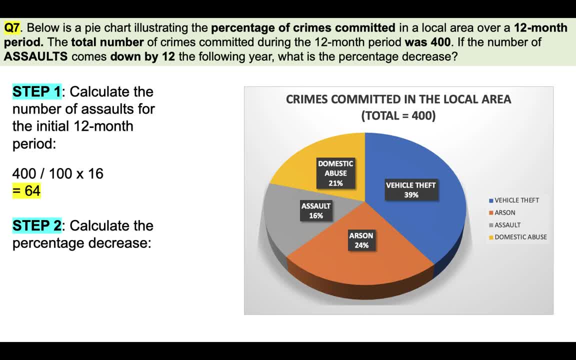 64.. Now, to calculate the percentage decrease, all we need to do is use the decrease number, which is 12,, because it's come down by 12, divided by 64,, which is the total number multiplied by 100, gives us the answer 18.75%. 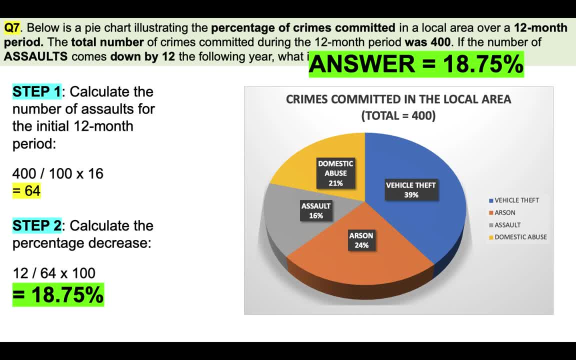 So if you just take a second to absorb that process, you can then use it to answer the question that's going to come right now. So you have to work out how to calculate the percentage decrease. So now it's your turn to have a go. Please put your answer to question 8 in the comments. 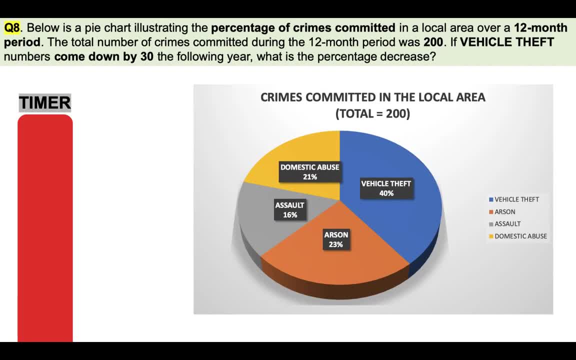 section below the video for marking, And your question is…. Below is a pie chart illustrating the percentage of crimes committed in a local area over a 12 month period. The total number of crimes committed during that period was 200.. If vehicle theft numbers come down by 30 the following year, what is the percentage decrease And 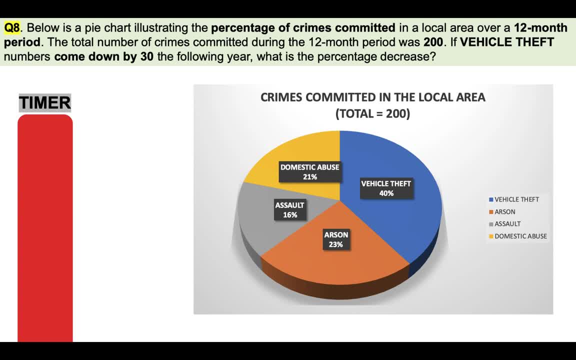 you have the time- It takes the timer to come down To put your answer in the comments section below. Here we go. Brilliant Well done. Let's move on now to the next one, And this is the question that I've been asking you for the longest time: How do you calculate the percentage decrease? 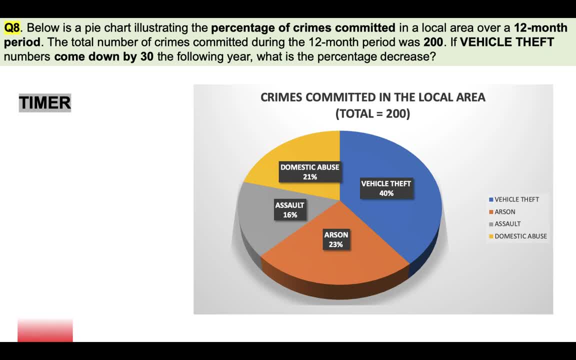 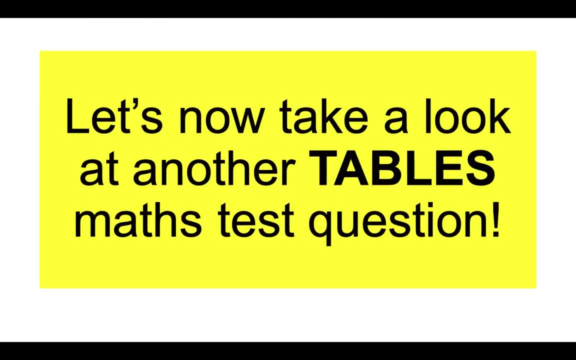 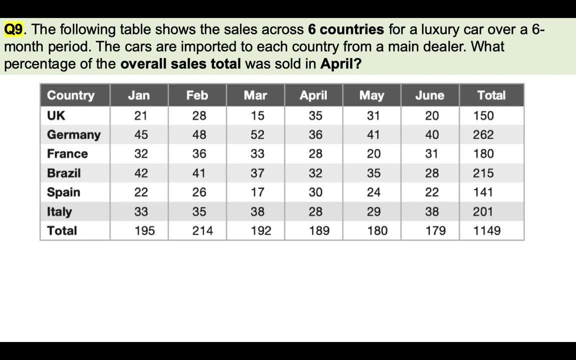 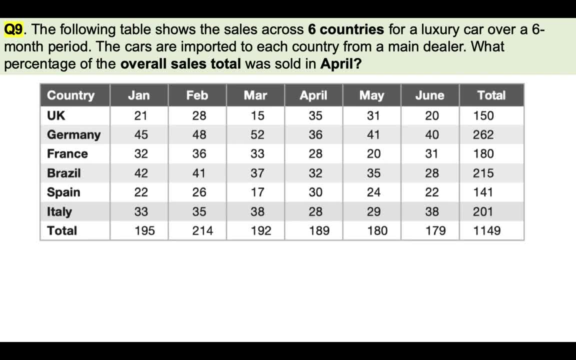 luxury car over a six month period. We've got January, February, March, April, May, June. The cars are imported to each country from a main dealer. What percentage of the overall sales total was sold in April? To tackle this question, step one- 189- is what? 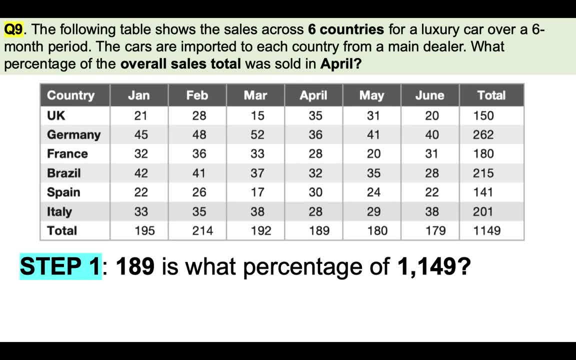 percentage of 1,149?? Because all we need here is these two figures, which is the April total figure and the total figure. We need to calculate what 189 is what percentage of 1,149?. To achieve that, all we do is 189 times 189.. 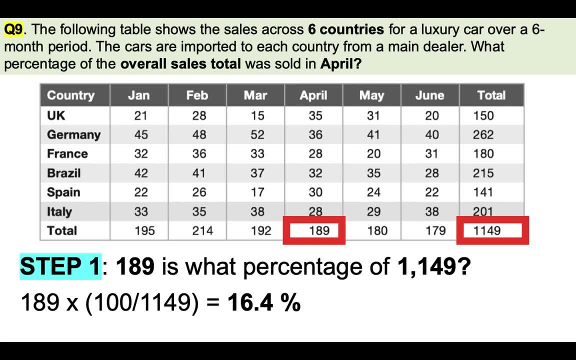 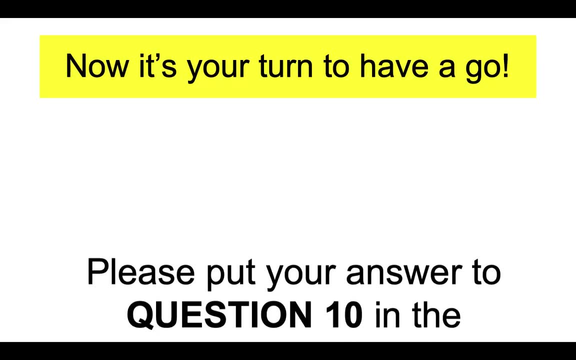 And we use a calculator to get the answer, which is 16.4%. Because the question is what percentage of the overall sales total was sold in April And the answer is 16.4%. So now it's your turn to have a go. Please put your answer to question 10 in the comments. 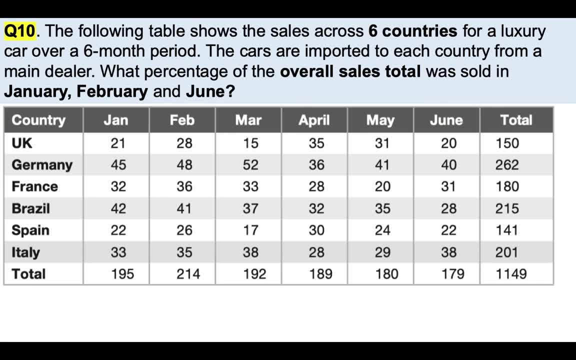 section below the video for marking. The following table shows the sales across six countries for a luxury car over a six month period. The cars are imported to each country from a main dealer. What percentage of the overall sales total was sold in January, February and June? Now I've not got a timer on this. 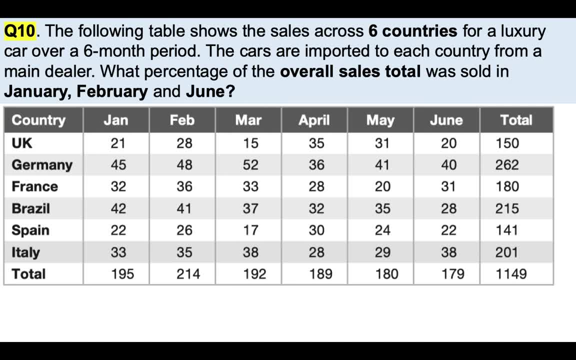 page because of the size of the chart that you need to look at, but I will count to 30 and tell you when that time is up. So what percentage of the overall sales total was sold in January, February and June? Here's your 30 seconds. 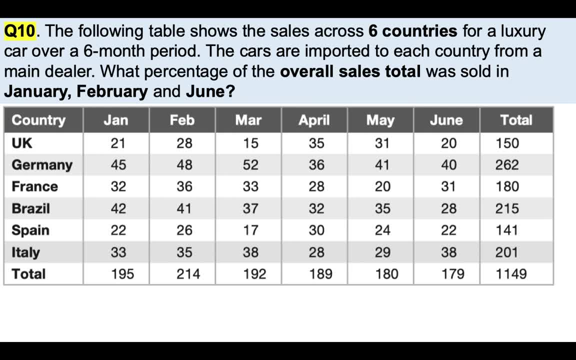 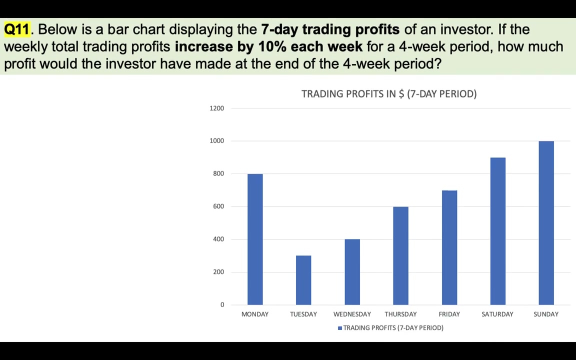 That's good. Okay, Brilliant, Well done. Let's now take a look at another bar chart. maths test question, Question 11.. Below is a bar chart displaying the seven-day trading profits of an investor. If the weekly total trading profits increase by 10% each week for a four-week period, how? 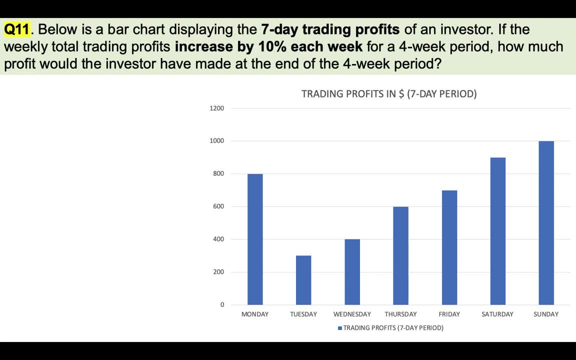 much profit would the investor have made at the end of that four-week period? So you can see here the title of the bar chart is trading profits in dollars for a seven-day period: Monday, Tuesday, Wednesday, Thursday, Friday, Saturday, Sunday, And then up that side on: 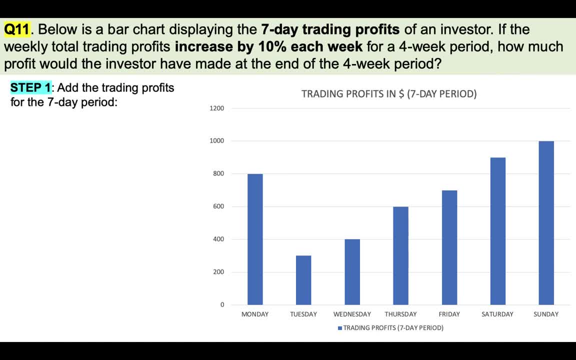 the left we have the totals. So to tackle this question, here's what we need to do: Add the trading profits for the seven-day period. In this case it's 800 plus 300 plus 400, plus 600, plus 700, plus 900 plus 1,000. And we would get $4,700.. Step two: add 10%. 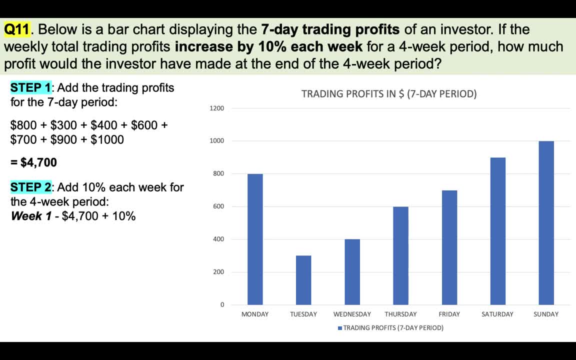 each week for the four-week period. So week one we have $4,700.. Add 10%, which is $470,, we would have $5,170. plus 10% of that is $5,608.7. plus 10% is $6,255.. Sorry, $170.. So step three: 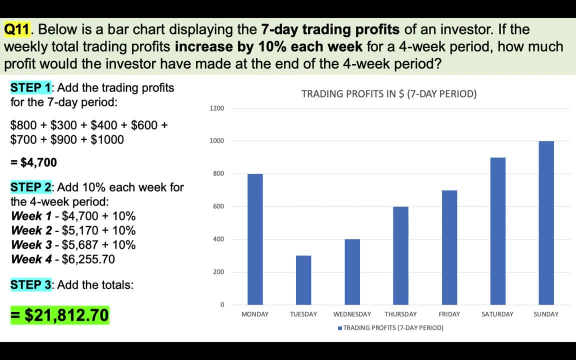 all we need to do is add all of those totals up and we get the total of $21,812.70.. $21,812.70.. Okay, So now it's your turn to have a go. Please put your answer to question 12,. 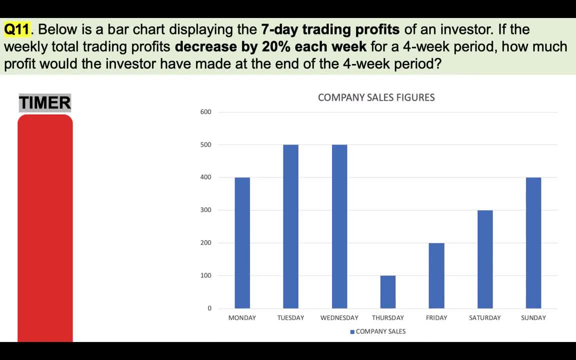 in the comments section below the video for marking. Below is a bar chart displaying the seven-day trading profits of an investor. If the weekly total trading profits decrease by 20% each week for a four-week period, how much profit would the investor have made at? 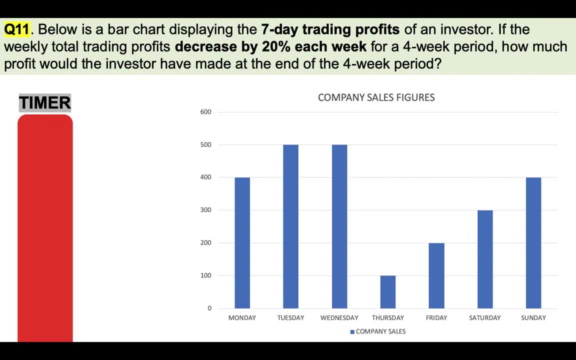 the end of the four-week period. So it's decreasing by 20% each week for a four-week period. When you have the time, it takes the timer to go down to zero. to put your answer in the comments section below. Here we go. 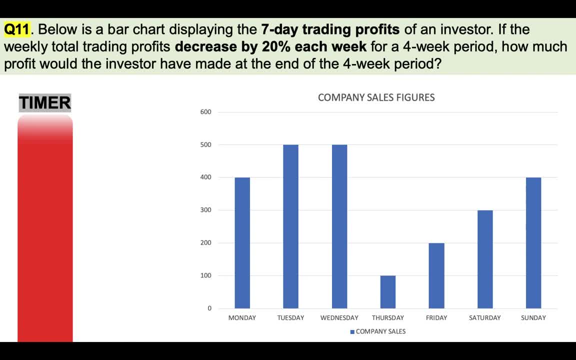 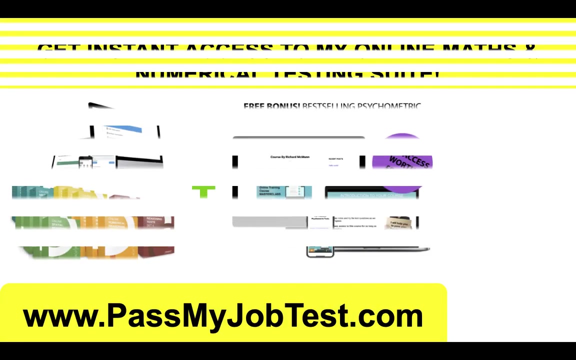 Thank you, Brilliant Well done, And you will notice that I gave you a bit more time because that was a more advanced calculation to carry out. So what I would like you to do now is, if you click that link in the top right hand corner of the website- sorry of the video-